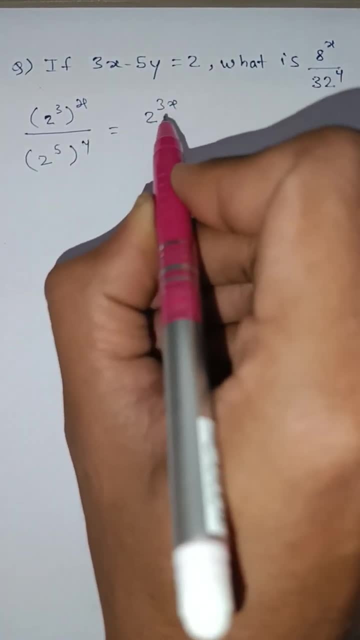 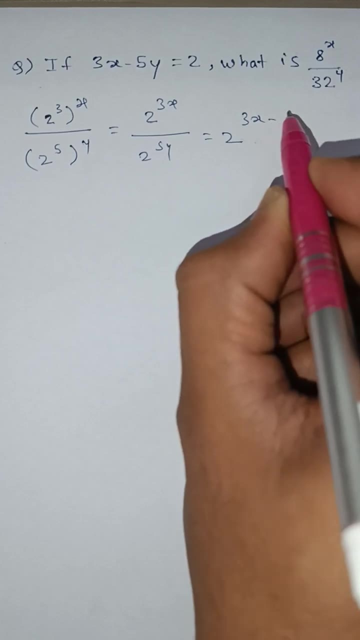 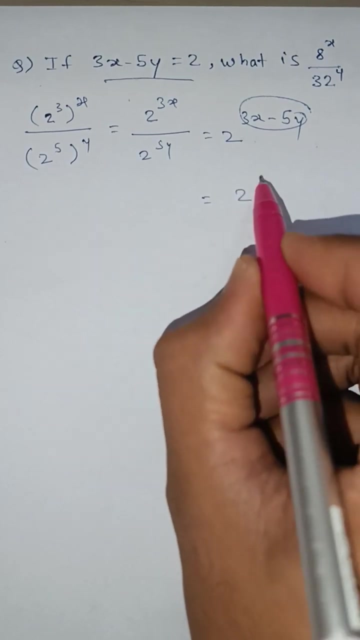 So this is 2 to the power 3x divided by 2 to the power 5y, which is 2 to the power 3x minus 5y, And this expression we know. the answer to It is 2 square, The answer is 4.. 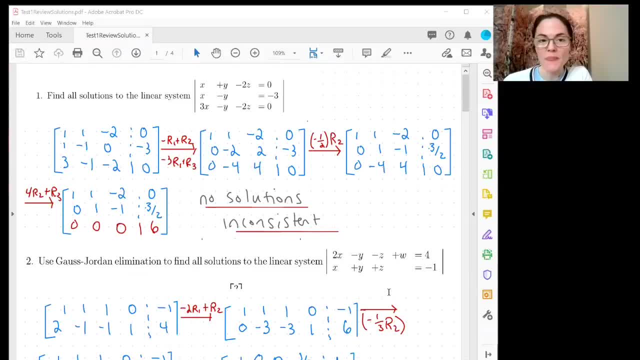 I'm going to go over the test one review. Most of the problems I will work out on the screen as I discuss them, except for the first two, I have them worked out already and I will talk about them, in part because we have probably the most practice with solving linear systems at this point in the semester. So let me just talk about the steps that I did. 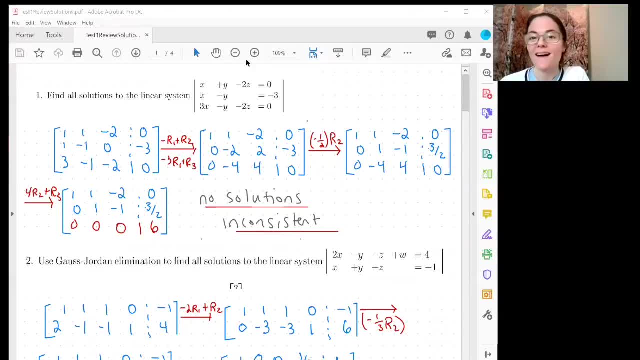 In number one. okay, let me also get this spotlight. Okay, wonderful, So in number one. my goal initially is these two entries underneath this: the 1, 1 position, which is already a 1, I want to make 0 so I can transform to reduced row echelon form: minus row 1 plus row 2 and minus 3: row 1 plus row 3.. 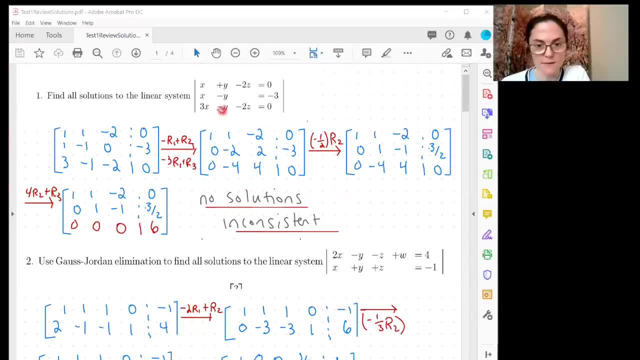 And the result is this: Okay, and then I'm good, I have zeros underneath this first one. I'd like to make this, minus 2 a 1.. This will be my second leading 1.. Okay, so I just multiply row 2 by negative a half. 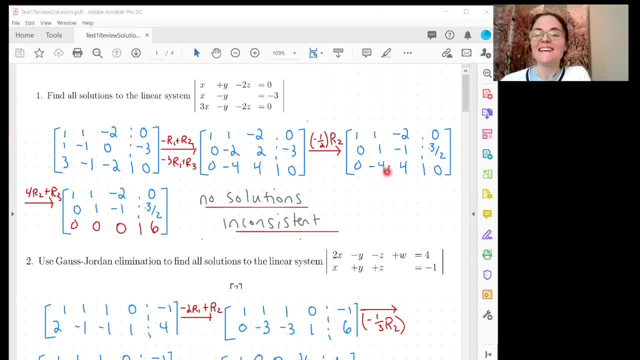 Okay, and then finally. well, the goal would be to get a 0 here and then work back up to get into reduced row echelon form. However, when I go to get a 0, okay, I take 4, row 2, add it to row 3.. What happens? I get this row of zeros followed by a 6 in the vector part. Okay, and this is problematic. Whenever we see a row of zeros, the dots something non-zero, immediately we know the system is inconsistent because, in effect, the last line, as it reads right now, says 0 equals 6, which is of course, not true.